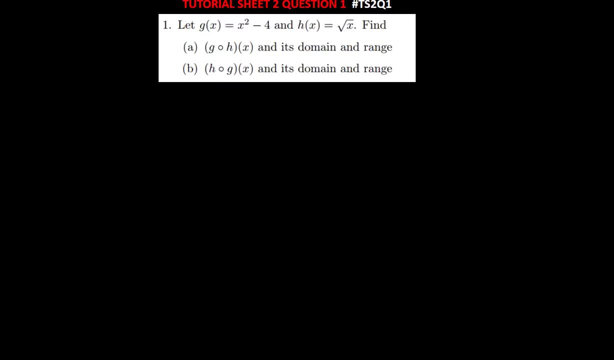 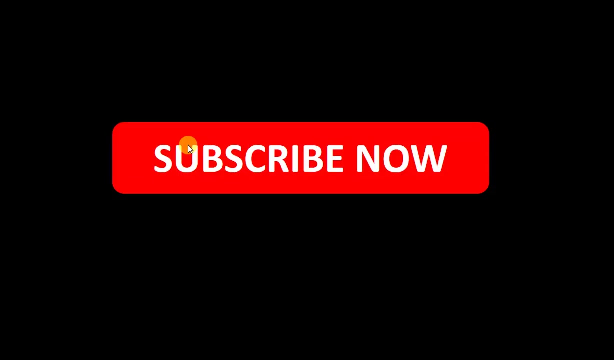 Hi everyone. so I come back with another tutorial. So today we are going to be solving a question from tutorial sheet 2, or beginning tutorial sheet 2 today. So this is question 1 from tutorial sheet 2.. So these questions are straightforward. Yeah, these questions are straightforward. Those that have not yet subscribed to my channel, please click on the button which says subscribe so that you don't miss out whatever that I'm going to be sending on the tutorial video. I mean on the channel. 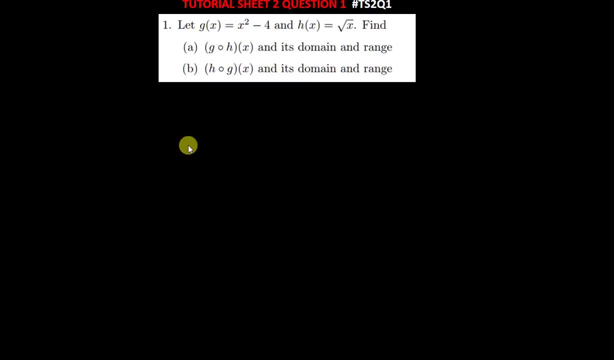 So this is this question is very simple. The question is saying: let g of x be equal to x squared minus 4 and h of x be equal to the root of x. Find a g of h, g of h of x and its domain and range. So here what you need to understand. you need to know what is this g of h of x. So these are what we call composite functions. 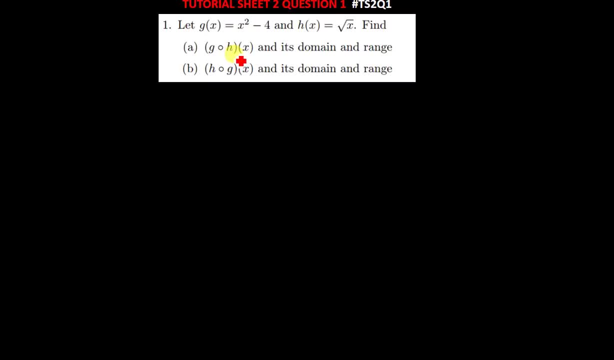 The definition of composite function, the simplest one is just a function in a function or a function within a function. So here, to start with, we're going to list our g, So our g, So our g of x, So our g of x is equal to x squared minus 4.. 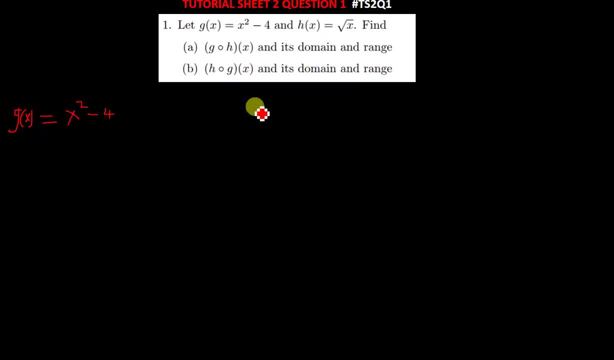 Our g of x is equal to x squared minus 4.. So here, if we've been taught, for instance, to find g of 1.. This is just an example I'm giving for for you to understand. if you've been taught, for instance, to find g of 1, you're going to say whether, wherever there's x in this expression, you put one, and they need to be like this. So here you get your answer to be negative 3. If you have been taught to find g of 1, you're going to say: whatever this x in this expression, you put one, and they need to be like this. So here you get your answer to be negative 3.. If you have been taught to find g of 1, you're going to say: whatever this x in this expression, you put one, and they need to be like this. So here you get your answer to be negative 3. If you have been taught to find g of 1, you're going to say: whatever this x in this expression, you put one, and they need to be like this. So here you get. 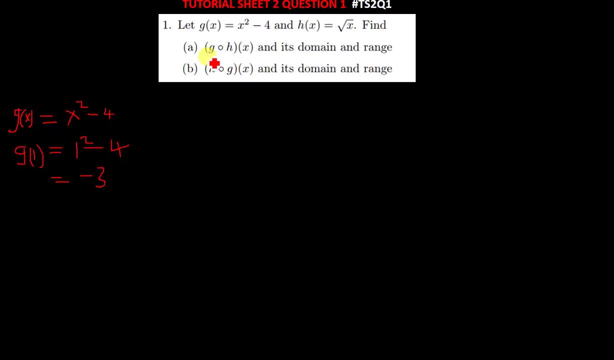 one. now, in this case they'll be. they have taught us to say find g of h. so meaning why there is x in this expression we're going to be replacing with h. so why there's x in that expression, g of one, we are replacing with one. now g of h. meaning whatever this x, we're going to put one. i'm sorry. 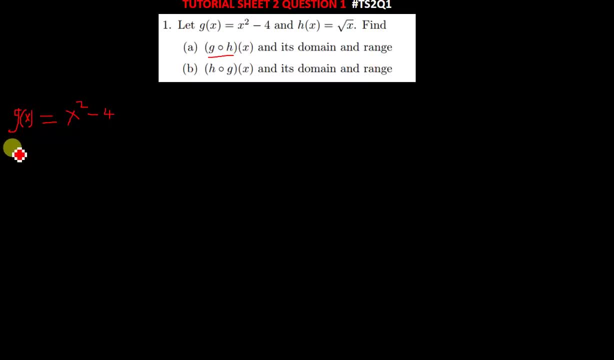 wherever this x, we're going to put h. so to find g of h, to find g of h of x, we just say: wherever there is x in this expression, we replace with what h minus four, like that. so this is my h. here, h is just equal to the root of x. so why this x? i'll put h there. 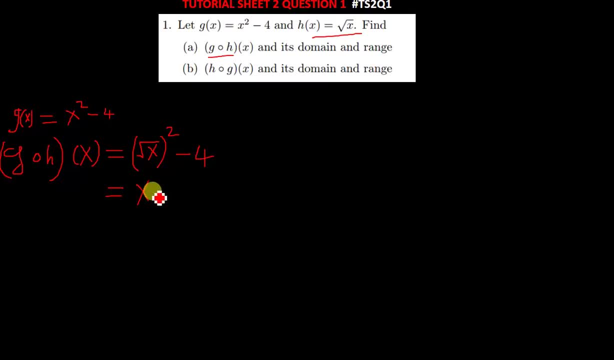 so i'm going to have my solution to be x minus 4.. so this is my first solution. so it's also going further to tell me to find the domain and the range. how do i find the domain? so the domain is just a set of inputs, the set of x values. so 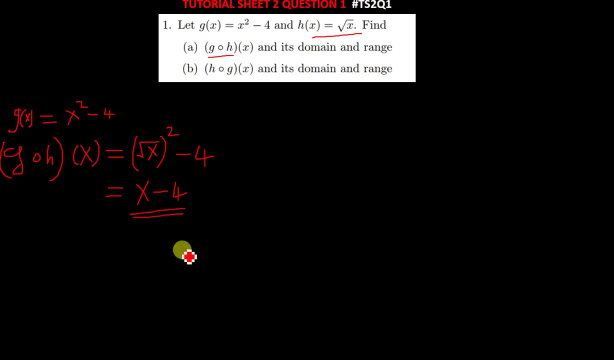 the set of inputs. here, in this question, there is no number, there is no real number. that can make this question undefined. hence the domain. the domain. it would just be equal to all real numbers. it's the set of all real numbers. if you want to write, if you don't want to write it this way, you 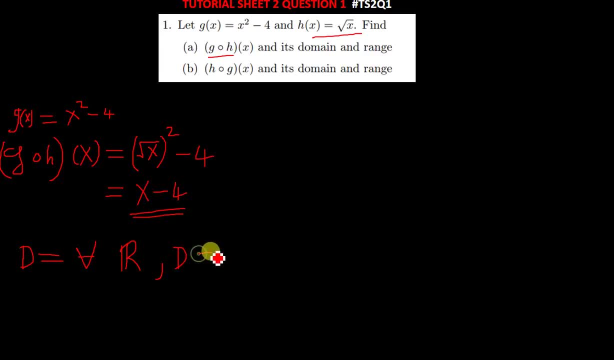 can just say: the domain is equal to the root of x, to a negative infinity, up to where infinity. this is the set for the domain. so you can either write it this way or this other way. all right, let's quickly move on to the next question. oh sorry. 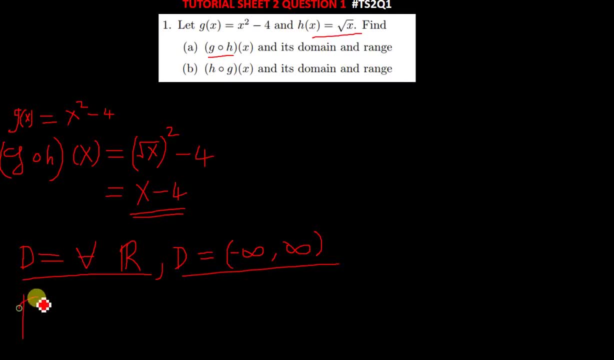 before we move on to the next question, we have to also to find the range. so how do you find the range? so when you replace all the real numbers there, what? what answers do you get? you? you still get negative. infinity to infinity, you still get this. we have no specific numbers that we are. 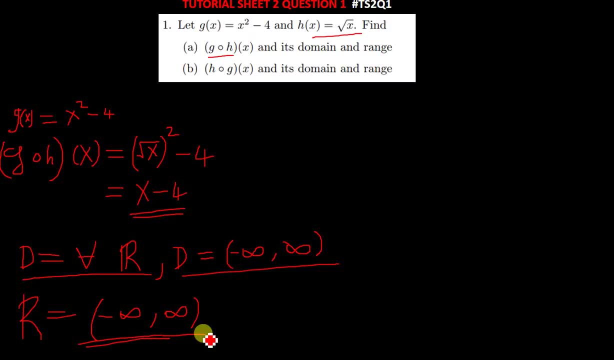 putting there we only have infinity. i mean from negative infinity to infinity, mean the range will also come out the same. all right, let's quickly move on to the next question. so the next question is saying h of g of x, so h of g, h of g of x, so meaning where there is x we're going to replace. 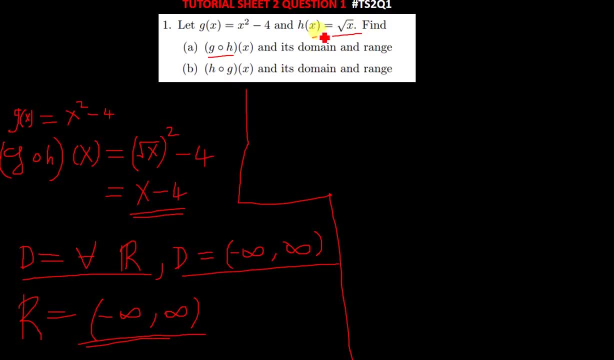 with h i mean with g in. in h where there is x, we're going to replace with g. in h where there is x, we replace with g. so our h of x has been given to be the root of x. so what is x here? we replace with x squared minus 4. so to find h of g of x. 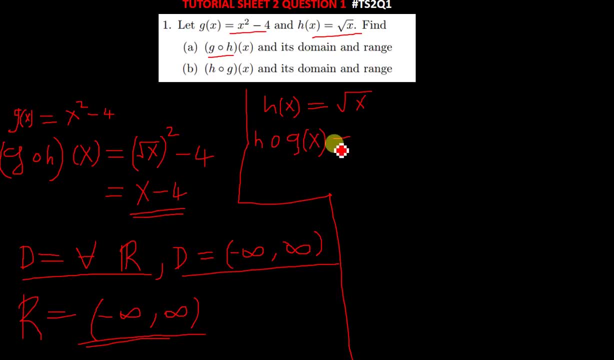 this is what we're going to have. we're going to replace here with x squared minus 4, where there is x. all right, so this is our h of g. so if this is the case now, let us try to find the domain here. now it becomes a little bit trick. 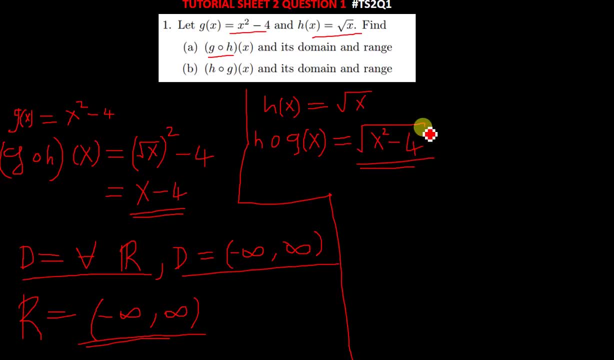 we have the square root here. this sad, this sad, this sad does not allow all the numbers to be inside there. here we're dealing with the set of real numbers. we don't want complex numbers. so here, to find the domain, we should avoid having complex numbers. so now, 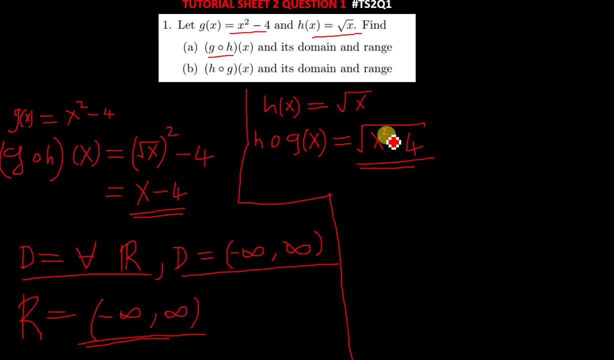 how do you find the domain and the range now? so to find the domain, the domain, all right. so to find the domain. here we can replace any number here, any number like, for instance: let's try to put zero there. when you put zero there, when you put zero at x, we're going to remain with negative. four: 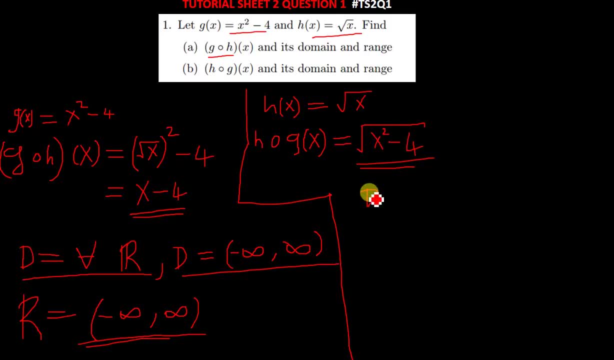 so zero, any number below zero, it i mean numbers, uh, number numbers like zeros, or they have done what denied us. we put one, it will still refuse. let us try to put two there. so when you put two, it's going to. it's going to do what it's going to be two squared minus four. 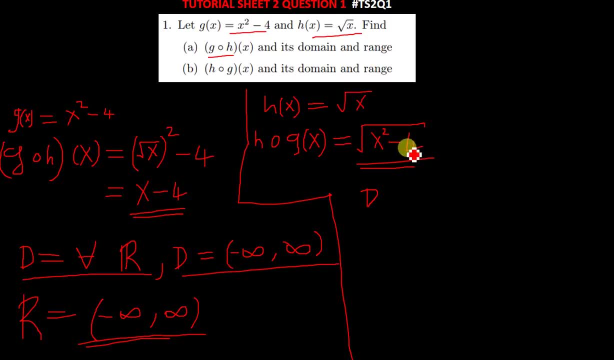 is zero. two squared is four minus four. it will give you zero. the square root of zero gets zero. so at least two has accepted. so if you want, or let me show you the simplest and easiest way to do this. so what you can do here, you just equate whatever that you have under the root there, you equate it. 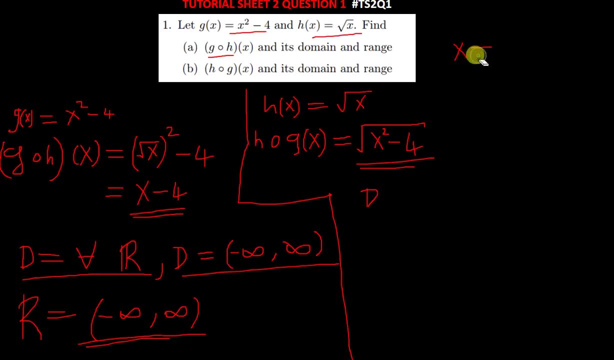 sorry, sorry, sorry. you get whatever that you have under the root to what to zero? you equate them to zero. so once you get them to zero this- oh sorry, not equating them to zero, but uh, you do watch this. you say this because we know to say whatever that we have here in the roots, under the root, here, whatever. 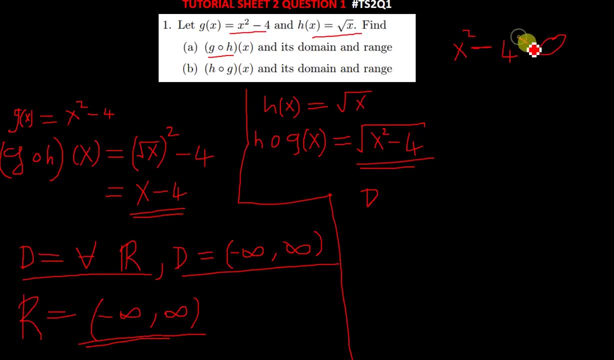 that we have under the root here should be greater than zero, not less than zero. if it's less than zero, then we're going to have complex numbers as our answer. so, whatever that we have under the root for us to have our answers to be real, numbers should be greater than zero. so what does this mean? so 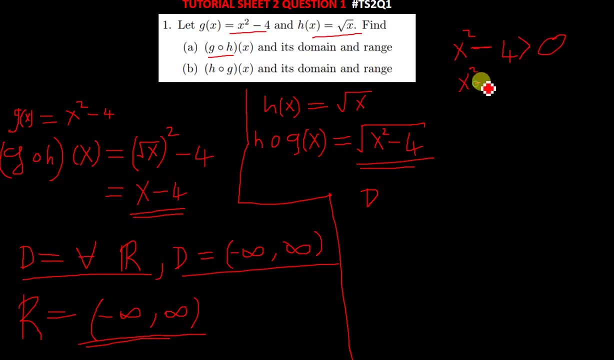 we're going to have something like this: minus two squared is greater than zero. yeah, so this is what we're going to have. so, when you look at this, this is a difference of two squares. it can be solved as x plus two, x plus two x plus two. 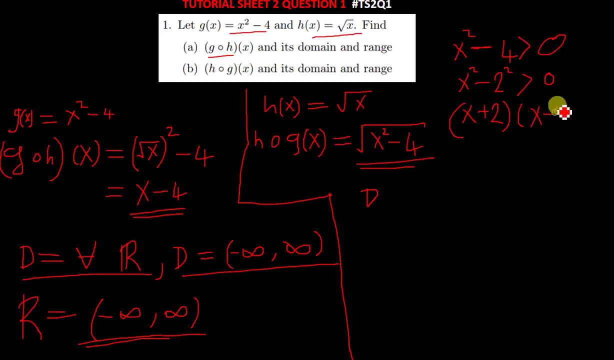 and x minus two greater than zero. so this is what we're going to have. so here the values of x are going to have. the critical points are going to give us x. when you get this, x plus 2 to 0, you get x is equal to. 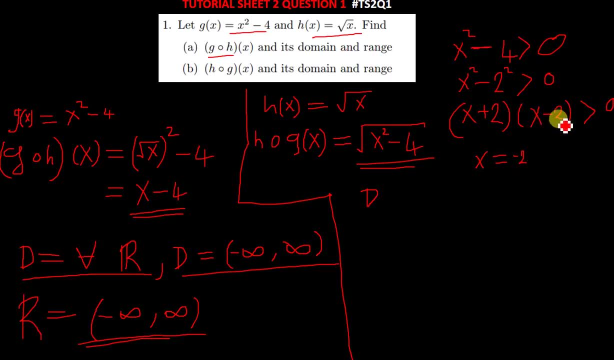 negative 2, and then, when you equate this x minus 2 to 0, you're going to have x minus. i mean x is equal to positive two. so these two values that we have here are the ones that we call the click, the critical points. so these critical points are the ones that we're going to use to find 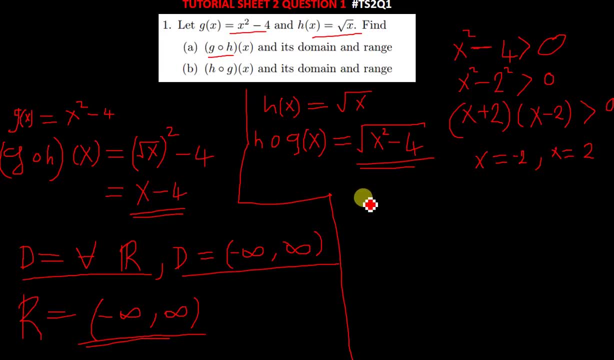 the domain. now, these are not the domains, but we've used them to find the domain. how do you do that? you draw a number line. so once you draw a number line, you're going to put your negative two there. you put your two there and then you put the ranges. so this side, we know that all numbers that are this side are- 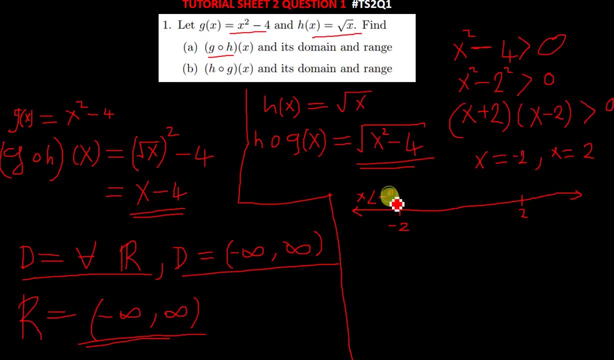 x are less than negative two. they are all less than negative two. and then numbers between here: between two and negative two. we know that, yes, they are between two and negative two, so you write them like this: this side, all the numbers are greater than two. so we begin to test the numbers. let's try to take any number that is, uh, less than. 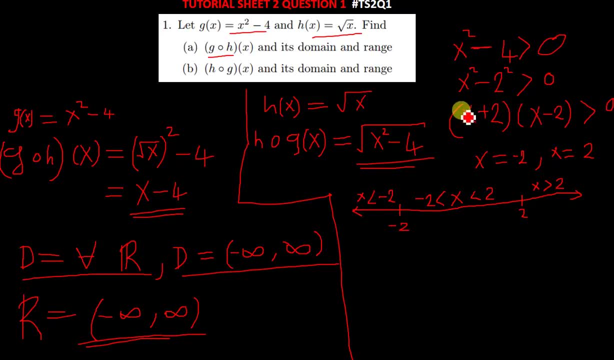 negative two, we put negative three. so when we put negative three there, negative three plus two, you get negative one. so i'll just write a negative there. negative three plus um a negative three minus two, you get negative five, i'll get a negative. you just get the same negative times: negative. 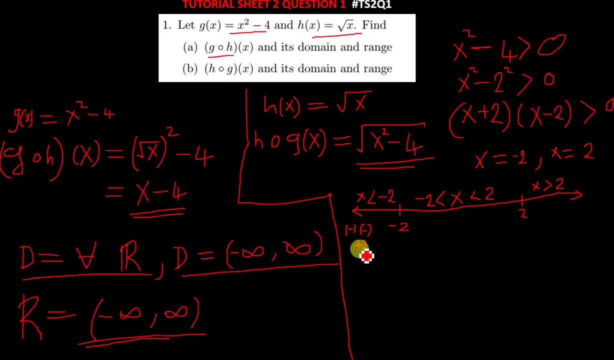 it's positive. so so this is. this is positive. now is a positive number uh, greater than zero? yes, so this part has accepted. let's get a number between negative two and two. let's write zero. when we get zero. zero plus two, get positive two. so get a positive number there. zero minus two, you get negative two. 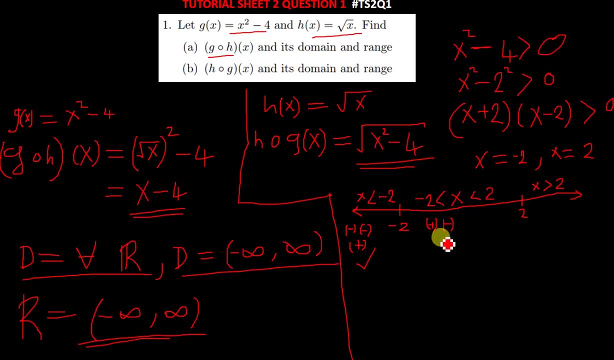 so you get a negative number there. when you multiply negative times positive, you get a negative is a negative number, so you get a positive number greater than zero. no, so this part has denied. we go to this other part. we get x grade: any number that is greater than two. we get three. 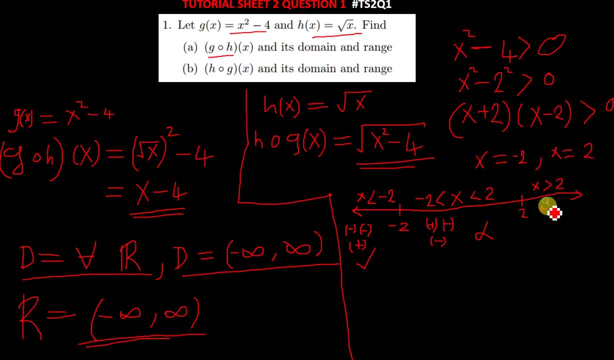 three plus two, you get a positive number. you write it there. and then three minus two, you get a positive one. you write it there. positive times: positive. you still get a positive answer. so is a positive number greater than zero? yes, so you mark it like so, meaning our domain is going to be equal to. so you just get these parts which you have marked. 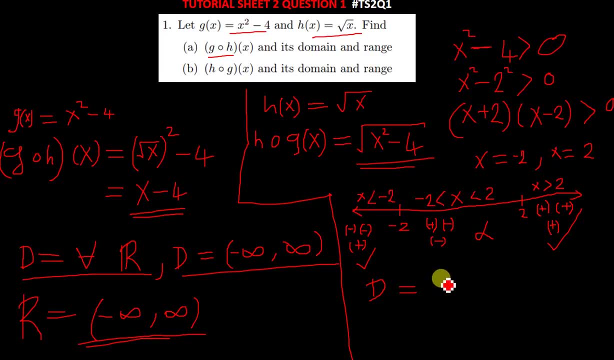 so meaning we have x less than negative two. so any number that is less than negative two can be put in that expression: any number that is negative that is less than negative two. so how do we write this in? uh, in interval notation: any number that is less than negative two, you. 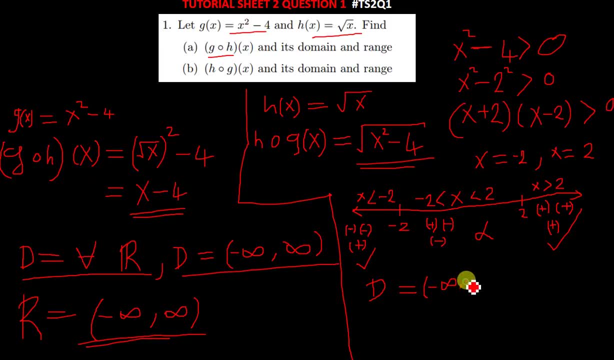 write it as from negative infinity up to negative two. yes, you do like that, wait. so here we said: this is supposed to be greater than. supposed to be greater or equal to, because even zero, ah no, supposed to be greater than, because when you put zero there, oh yeah everything that is under the root. there should be greater. 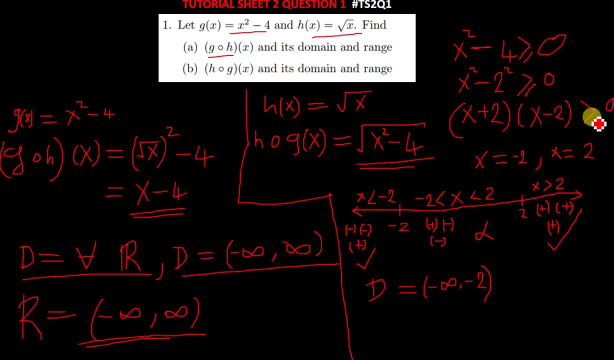 or equal to zero, so i i forgot to put a, an equal sign there. so here, man. so so here it's going to change. now, instead of using this bracket, we're going to use this, so even these signs there will change. we're going to have something like this: 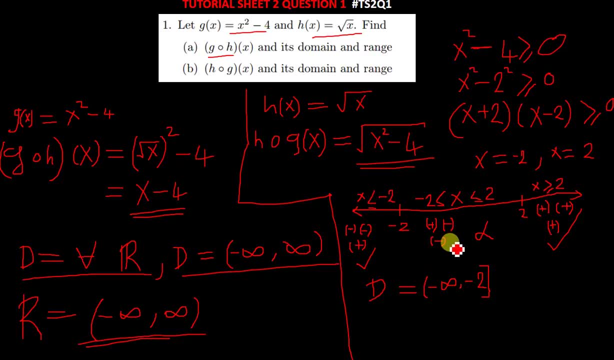 yeah, so this is going to be greater or equal to. why have i said greater or equal to? because we know to say even zero. here is, uh, a real number that is going to accept us there. it's going, it's going to deny, it's not going to give us a complex number. so why have i included this negative two? 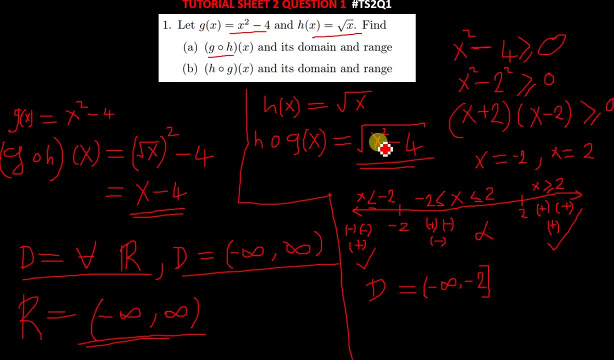 when you put negative two there, where this x to be negative two squared, you get four. four minus four, you get zero. the square root of zero is zero, so that one at least has given us a real number. so let us combine it with this other, so union. 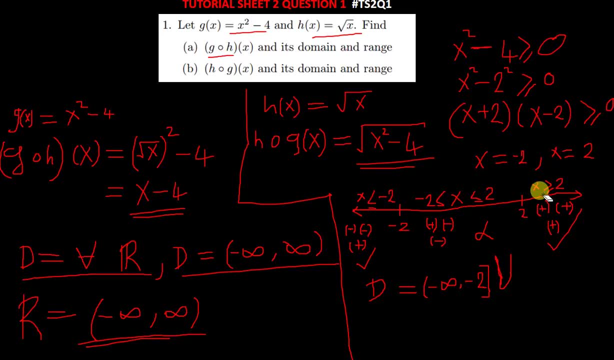 this part here. so how do you write that part in set builder notation? so that part in set builder notation is also. you write it, uh, also, as. so this is going to be x greater or equal to two. so it's going to start from where? from two up to where? positive infinity, yes, so this is it. 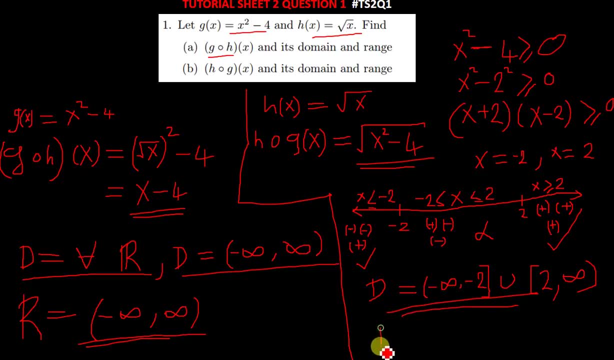 so this is your domain. now how do you find the range? how do you find the range? the range is simply the set of. uh yeah, so the range is simply the set of. so let me just do this. so domain is equal to that. so the, the values of the domain, are simply x values. so normally you say: 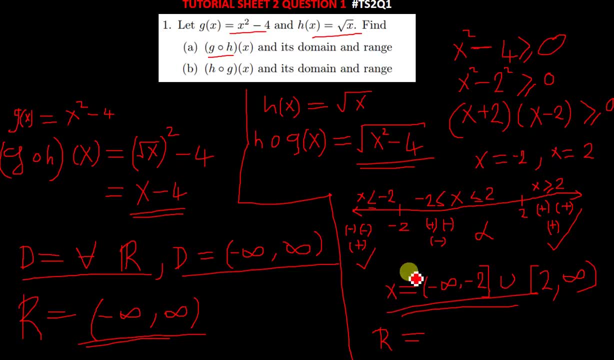 x is equal to this. so this is. these are the values of x. so let me just put them in brackets. so this is our domain, yeah, and then what is the range? yeah, what is the range. so, if you want, you can write it this way or the way that i wrote it. 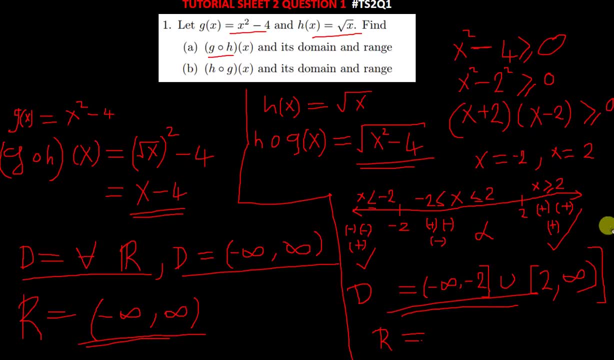 at first it is. it is still the same. they'll still make you correct, or you just leave it like this: d is equal to that. they will not to say it's a set of x values. and then we move on. what is the range? how do you find the range? so? 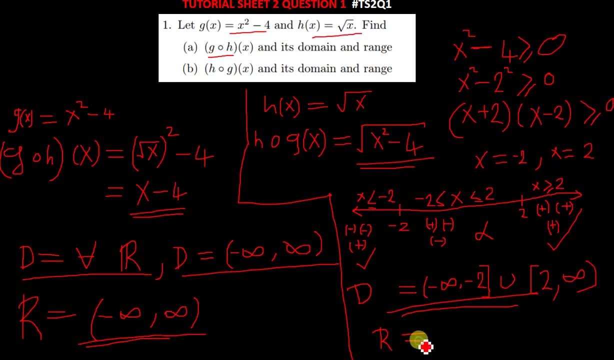 the range is gotten from the domain, so the the the worst is when you get, uh, any negative number there, any negative number less than two, you replace it there. what answers are you going to get? you get a positive answer, isn't it? so the same applies when you get any number greater than two. 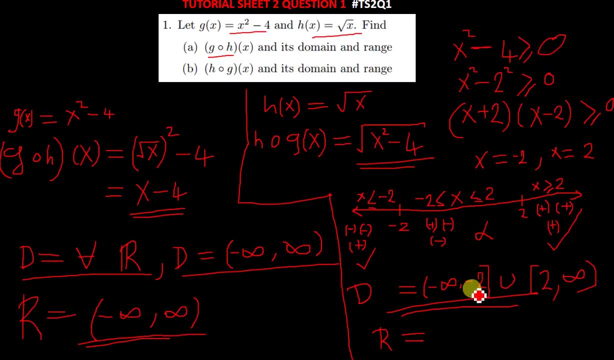 you get a positive answer. if you, okay, let's try to get two, first two. when you put two there, we're getting four minus four, which which gives us zero. the square root of zero is still zero, so meaning the smallest range value that we're going to have is zero, and then the highest value of the 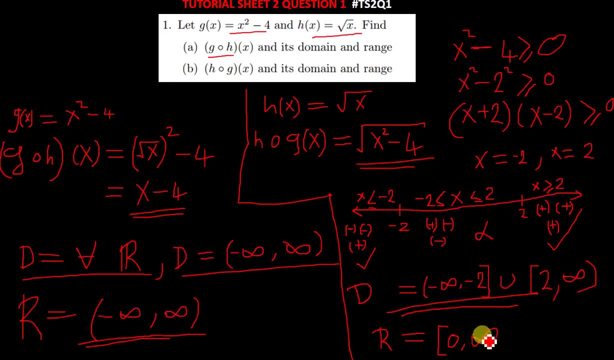 range that we're going to have is infinity. yes, it's not possible for you to get a negative number from there. hence, this is the range. all right, thank you very much for watching today's uh tutorial video. uh, please make sure that you subscribe to my channel. yeah, so this is the beginning of uh tutorial sheet two. 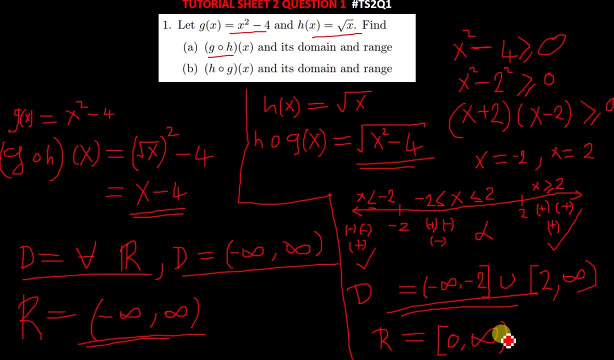 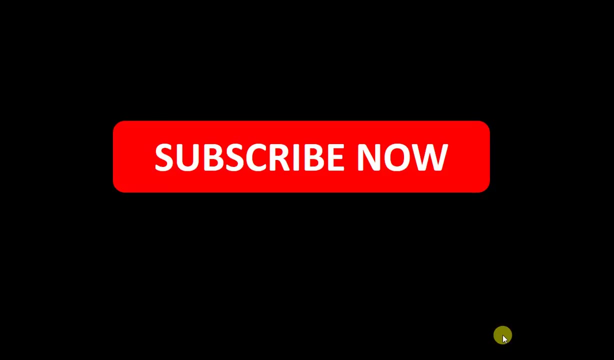 i'm going to also post the tutorial sheet. uh, two question, two answers. so this is just question one. yeah, this is just question one. so please make sure that you subscribe to the channel so that whatever that i'm going to be posting here you don't miss out. thank you very much for watching shalom. 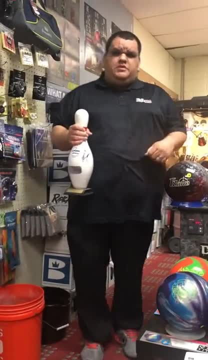 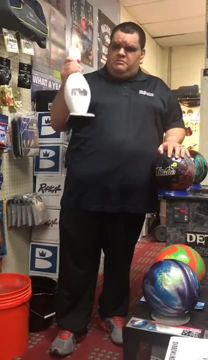 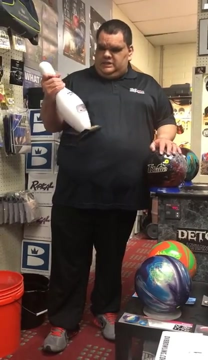 Hey guys, James Graham, here again from Double J's Bowling Supply with another vlog video for you guys, And today we're going to talk about weight and how important it is in a bowling ball. So this is a bowling pin. This is an award that was given to my brother for shooting 8.32 back on 3-9 of 18.. 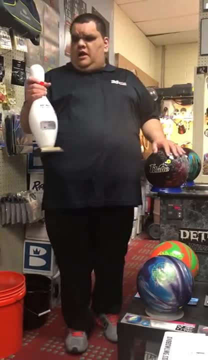 It was also signed by one of the greatest of all time, Norm Duke. A bowling pin weighs 3 pounds 6 ounces, So when you're talking about 10 pens back there, that's 36 pounds of pens. So you need about as much weight as possible to be able to throw that bowling ball about as fast as you can or with moderate speed to be able to knock down as many pens as you can. 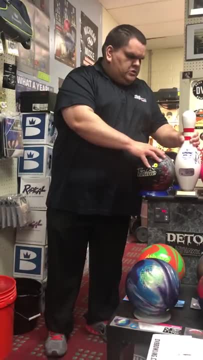 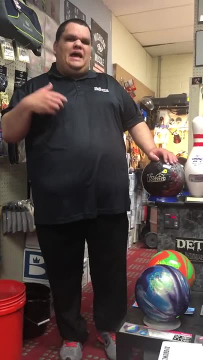 You know, very many times when I get people that come in the pro shop they always want to know: well, what weight should I use? Well, there's two kind of two main things to kind of look at, And first is kind of a fallacy, but I'll kind of tell you guys anyway. 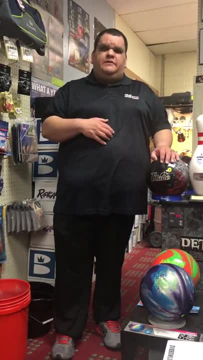 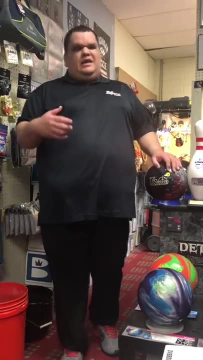 First, it's usually dependent on somebody's weight. It's usually 10% of somebody's body. Well, unfortunately they don't make a 30-pound bowling ball for somebody like me, over 300 pounds. The next, and that's kind of the fallacy there: